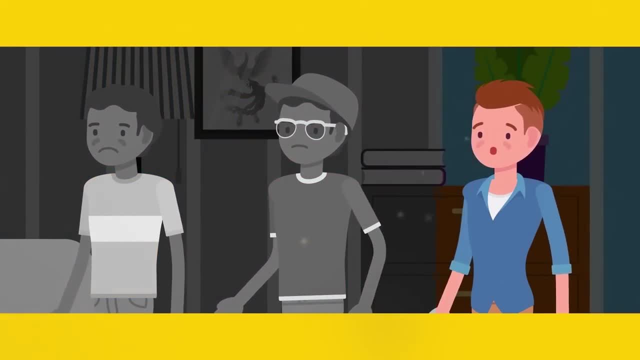 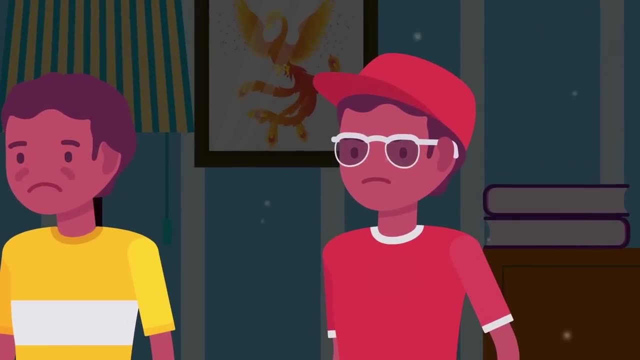 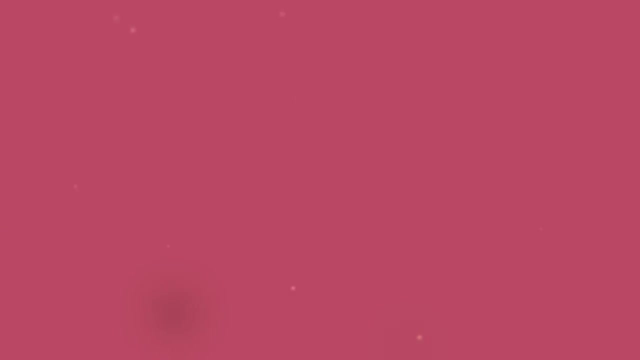 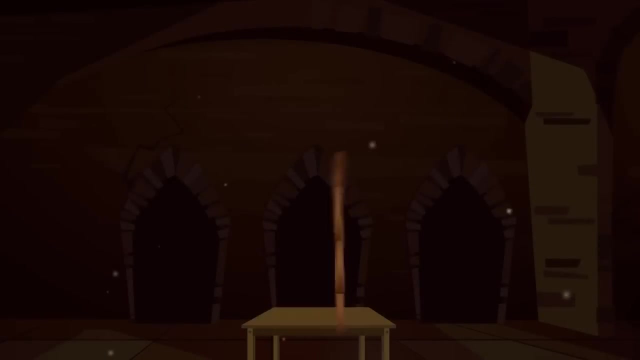 Who's lying, David? If he was allergic to cats, he wouldn't have lasted with Mia's cat in the same house for several months before You went to visit an abandoned castle, when you got trapped in the basement There's a small bamboo stick on the table almost as long as your forearm- In front of you. 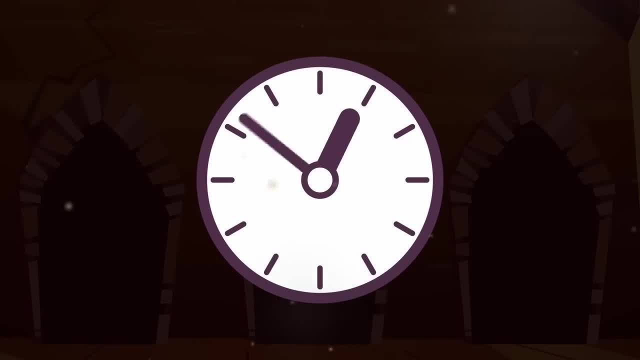 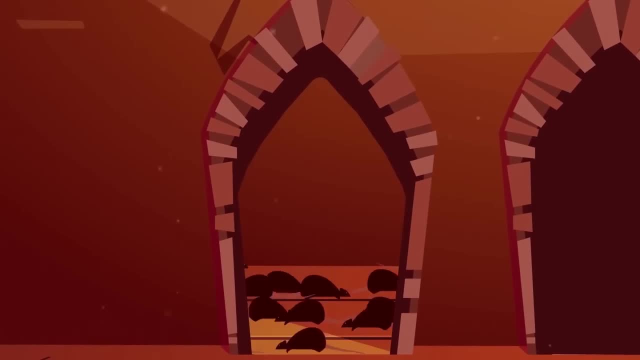 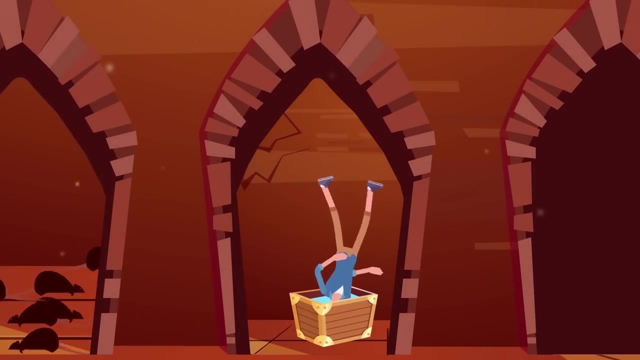 there are three doors and you must spend one hour behind one of them to get out of the castle, Which is the safest option. Behind the first door, there's 100 rabid wild rats. Behind the second, there's a box filled with water and you must keep your head submerged. 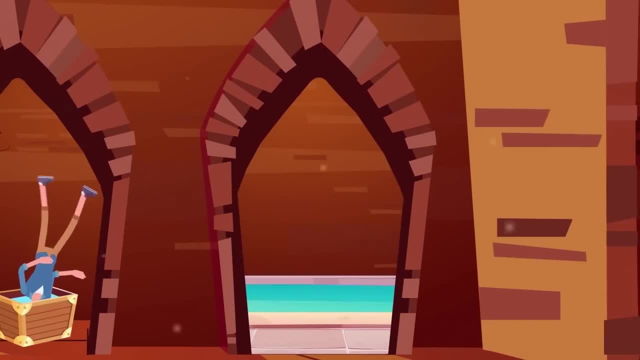 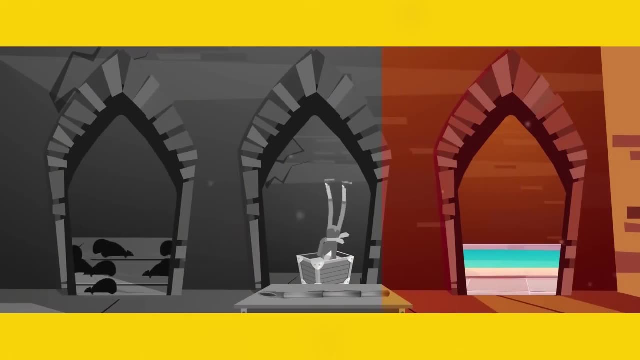 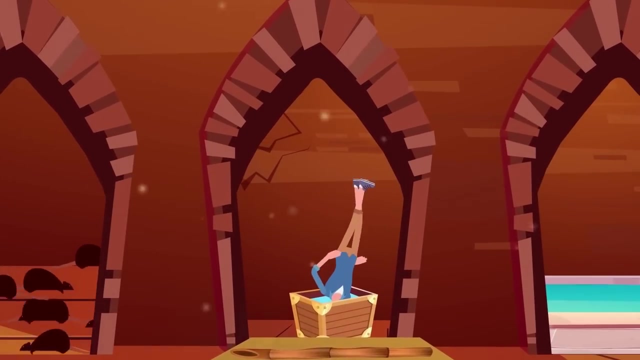 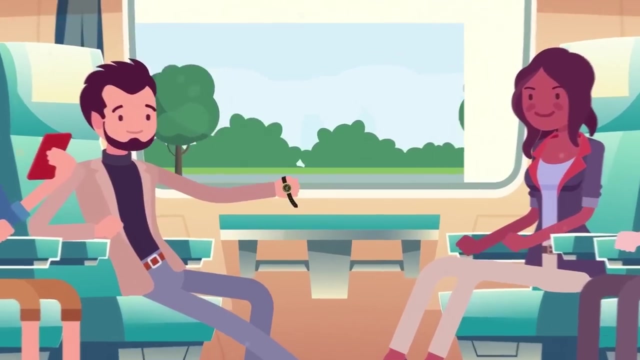 in it. In the third door there's an infinitely deep pool filled with box jellyfish. The second door: You can use the bamboo stick to breathe. Brian was traveling by train to a nearby city. He placed his watch on the table and was looking. 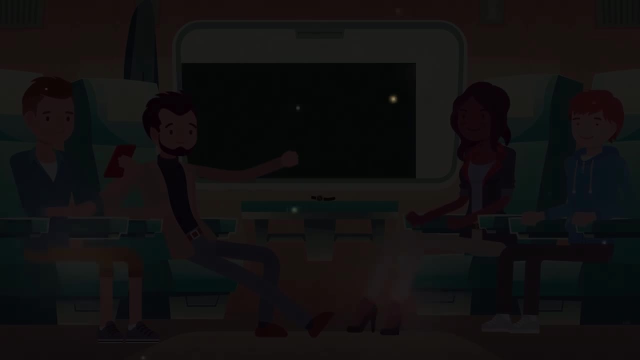 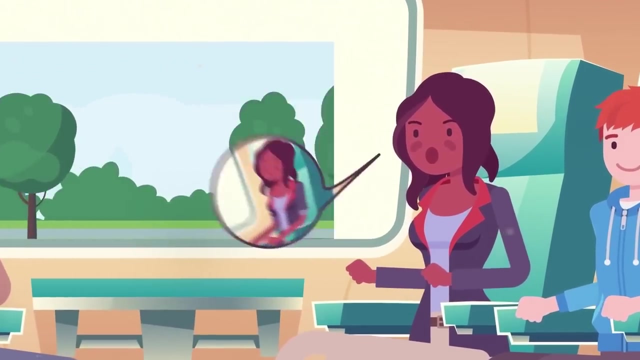 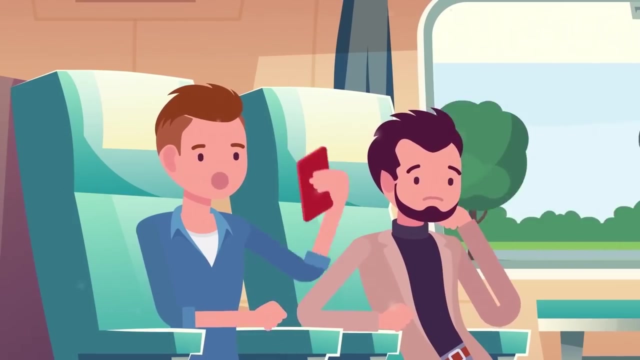 for his train ticket when the train went into a dark tunnel. When it came out, Brian's watch was gone. There were only three people in the car. Mary was sleeping the entire time. Christopher was looking for his wallet to grab a cup of coffee. Mike was playing a game. 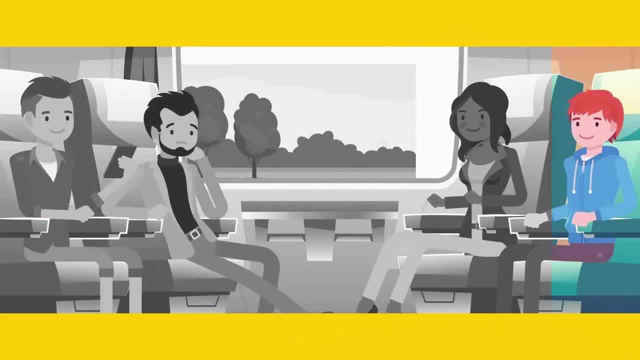 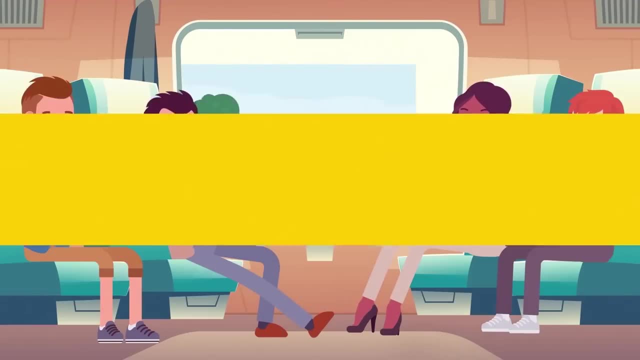 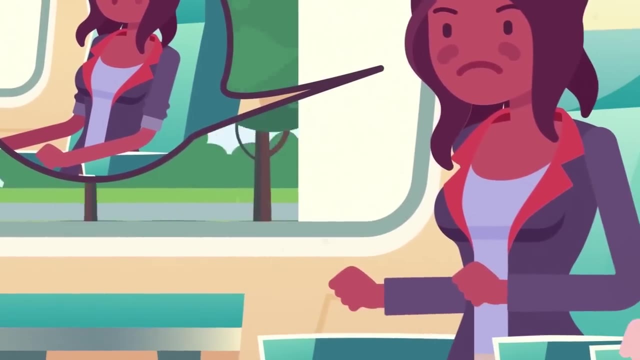 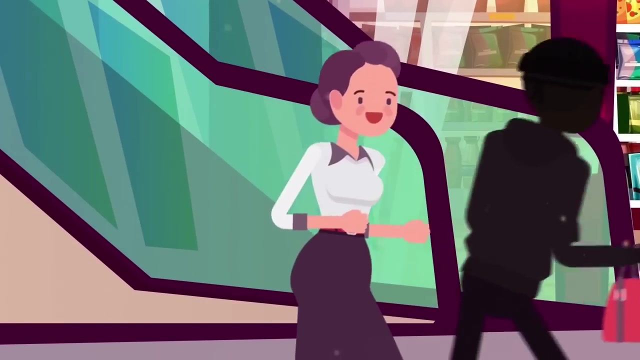 on his phone. Who took the watch? It was Mary. When the journey started, she had her sleeves rolled up and if she were sleeping she wouldn't put them down. Sarah was walking out of the mall when someone snatched the purse out of her hand and drove. 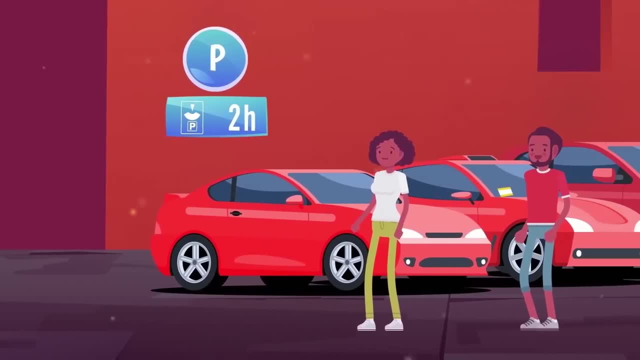 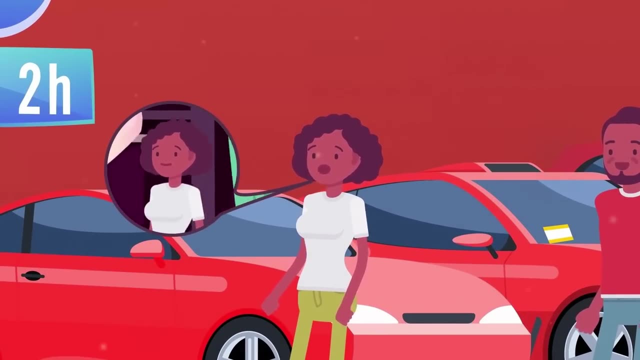 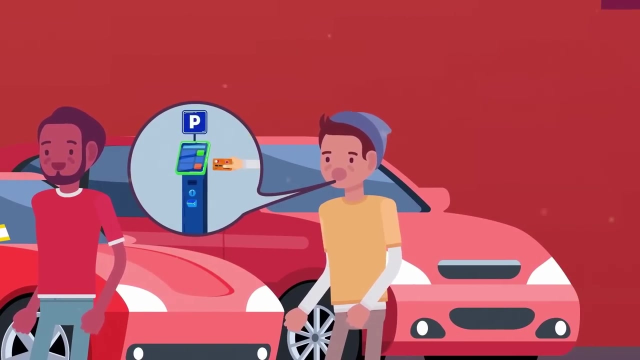 off in a red car. The security closed the parking lot and found three people with red cars. Alyssa said she was inside shopping when she got called by security. David said he had only just arrived. Bob said he was about to pay his parking fee and drive off. 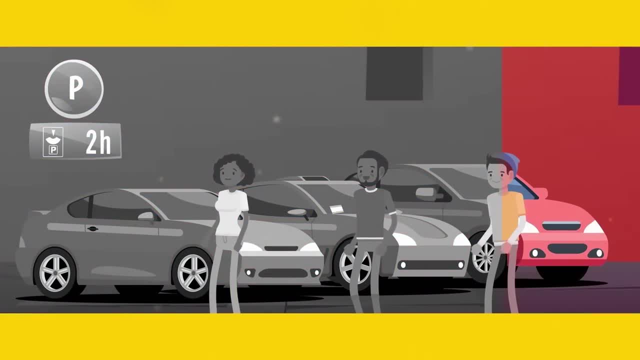 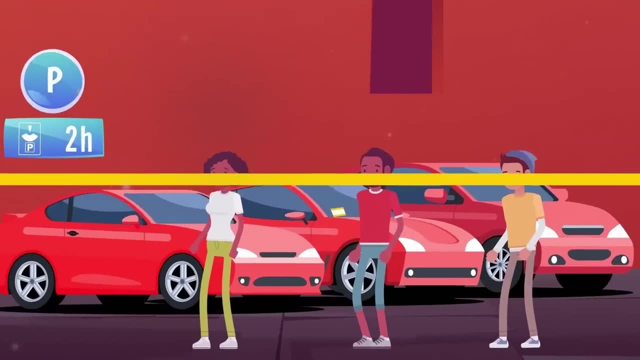 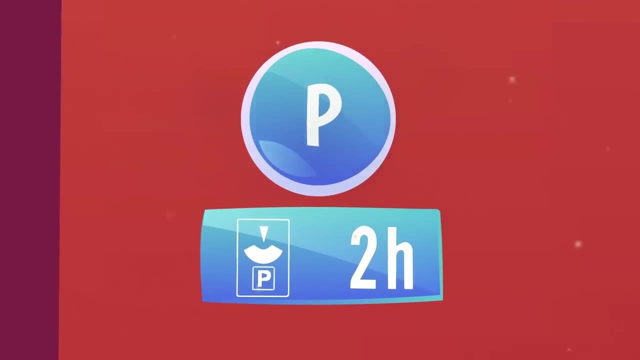 Who isn't telling the truth? David, He's got a room on his table and tires on the wall for more than two hours without paying and got a parking ticket. Whoever is telling the truth isn't a can of spirit Over, No. 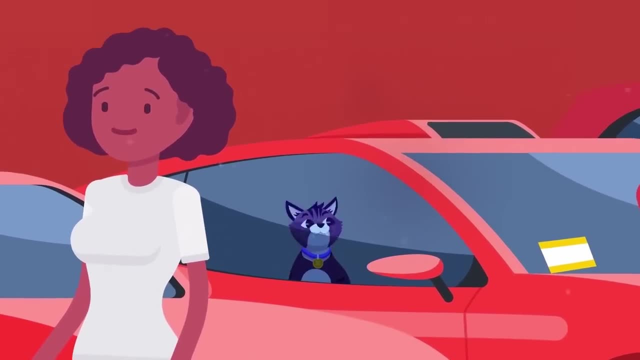 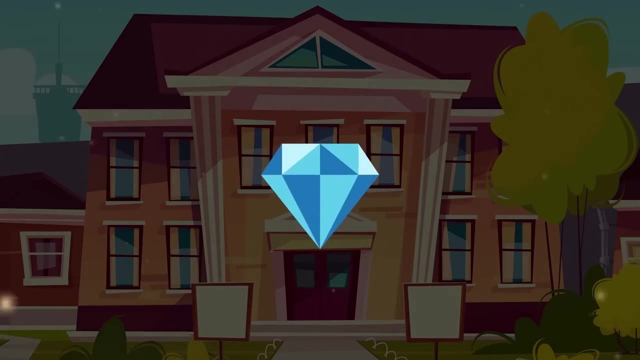 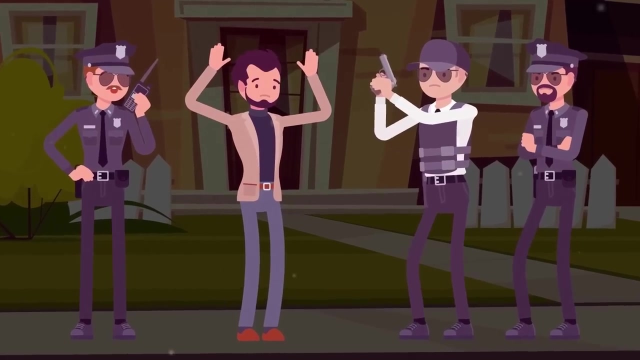 got a ticket And he lies about being very allergic to cats. Simon broke into the richest house in the neighborhood and took a very expensive diamond. Security guards caught him walking out and searched him for the diamond. They knew he'd taken it, so when they couldn't, 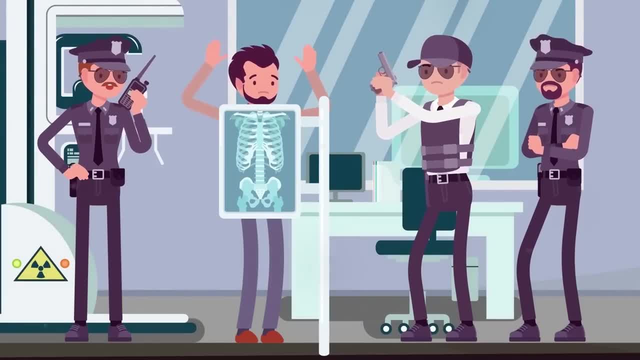 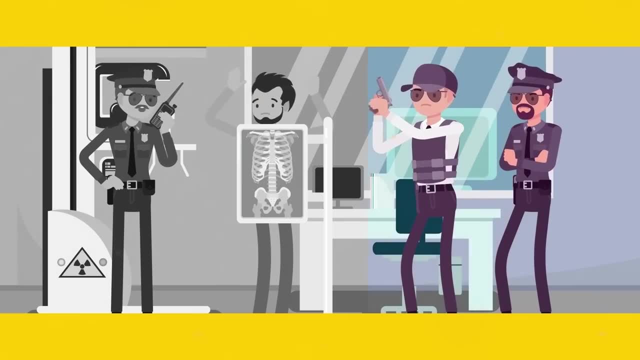 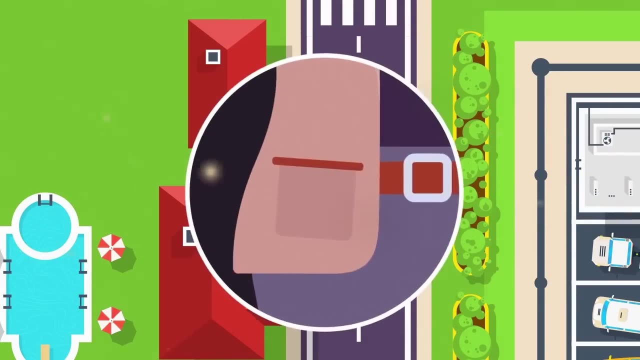 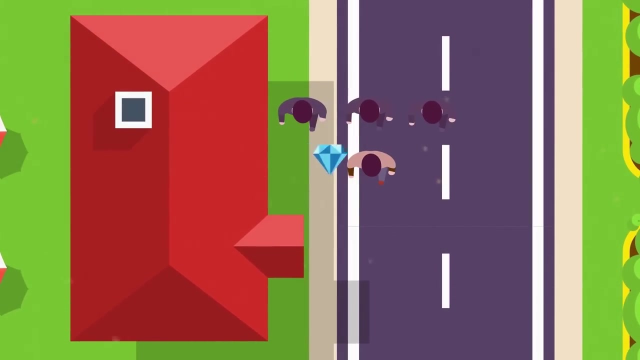 find anything. they x-rayed him. Still nothing showed up. Where was Simon carrying the diamond? As soon as the guards caught him, he put it in one of their pockets. After the search was over and they were driving him home, he took it out of their pocket with nobody noticing. 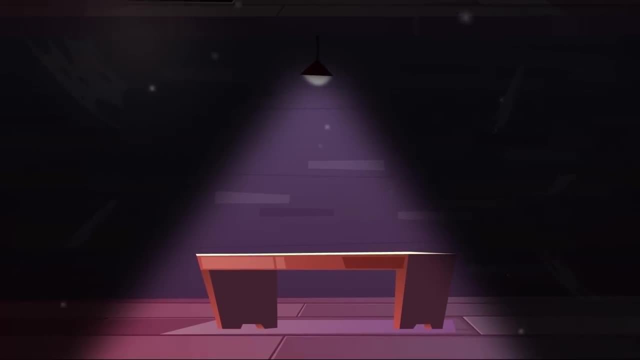 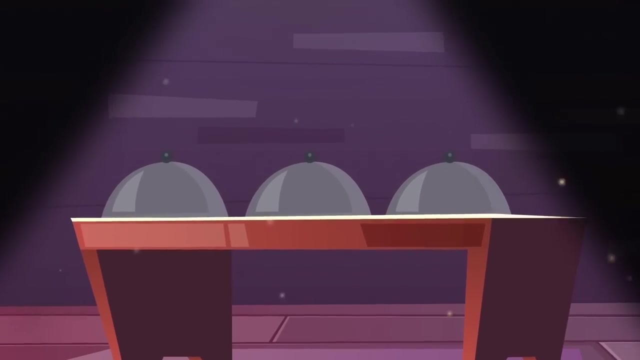 A crazy scientist took you into their basement and is planning to keep you there for a year. He's given you the option to choose one of three foods to eat for the year to stay alive. Which one do you choose to save your life? Pasta and bread. rice and beans, steak and broccoli. If you only ate pasta and bread, you'd get scurvy in just 8 months, And steak with broccoli is low in carbs, which will start breaking down your muscle mass to help you stay alive. 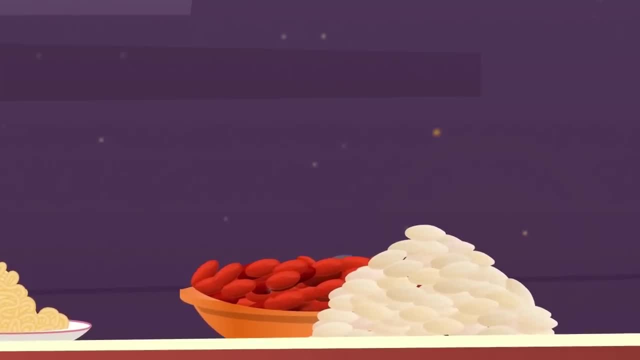 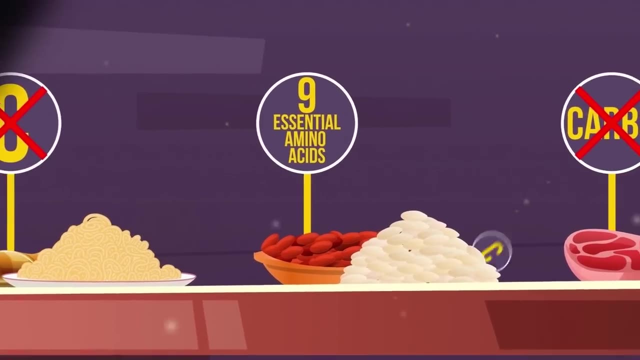 Your best bet is rice and beans. It's high in all 9 essential amino acids your body needs and you'll be fine. You can germinate some of the raw beans, eating their sprouts to get your vitamin C. Aren't you a smart cookie. 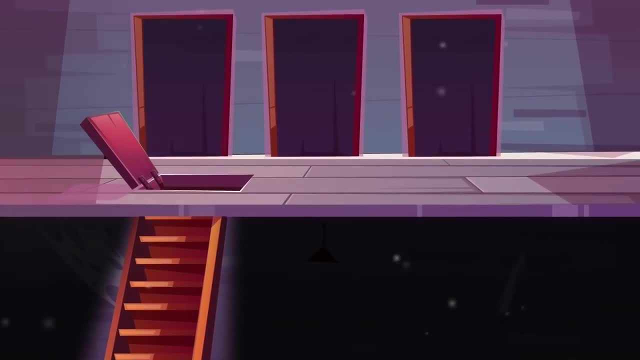 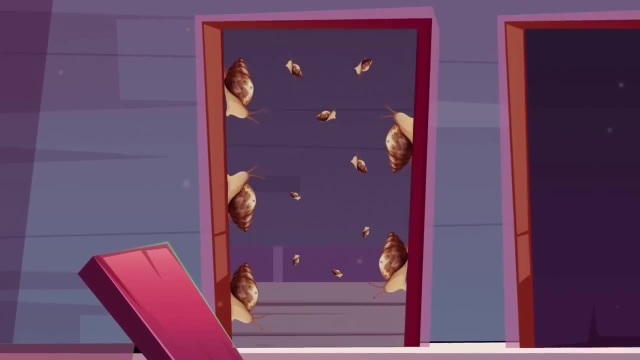 A year passes and you've managed to get out of the basement. But to make it out of the house you must pick one of the three doors the scientist created. The first room is filled with venomous cone snails. The second has 5 very hungry polar bears. 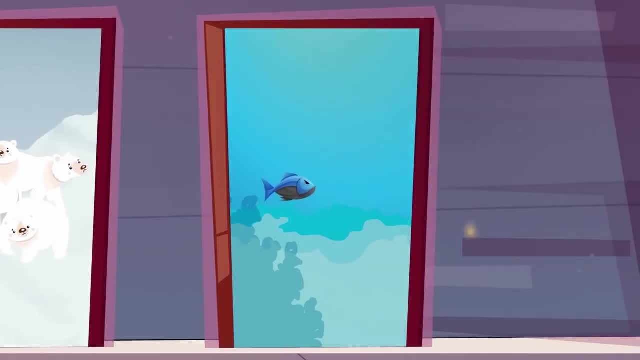 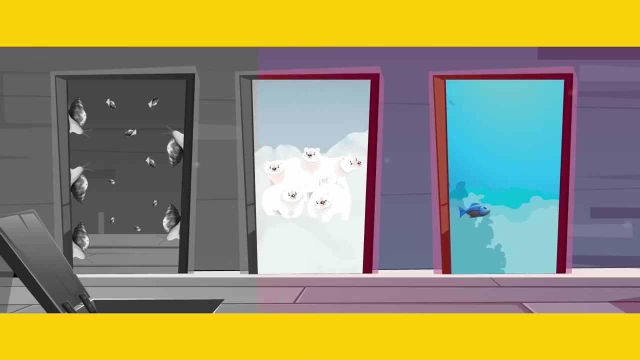 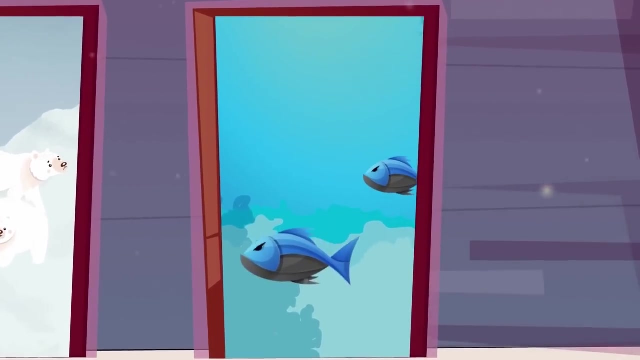 The third is a saltwater tank with hundreds of piranhas, Which is the safest. The third room is filled with the most dangerous live-d [ fish from the African desert. The third room: Piranhas are freshwater fish and can't survive in saltwater. 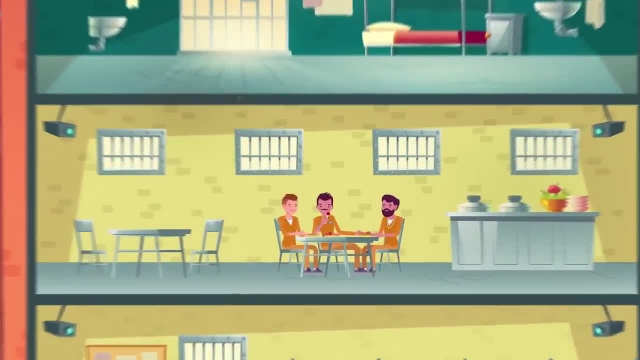 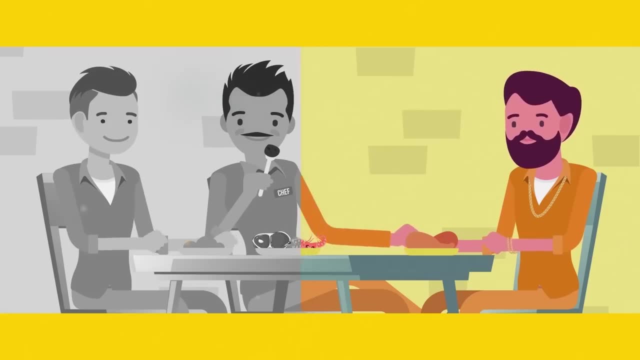 Three prisoners are sitting at the table having dinner, But one of them is wealthy. Can you guess who it is? The first room is full of creatures saved by the scientist, The second is full of creatures saved by the scientist And the third is full of creatures saved by the scientist. 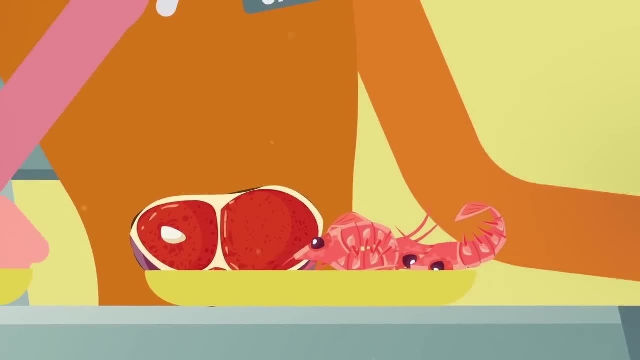 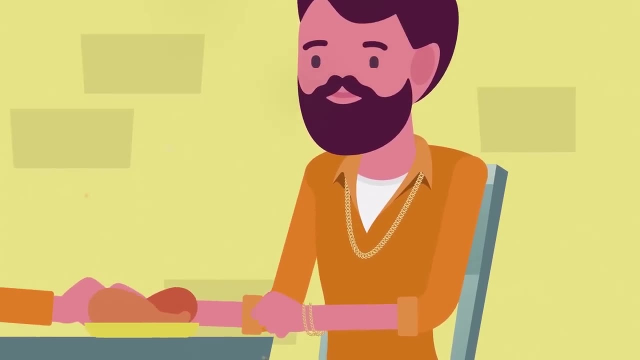 It's not the guy with the steak and the shrimps. The little tag on his shirt reveals he's a chef and he likes to prepare a special treat for himself. The guy with the jewel shows that he's rich, but in prison jewelry is basically worthless. 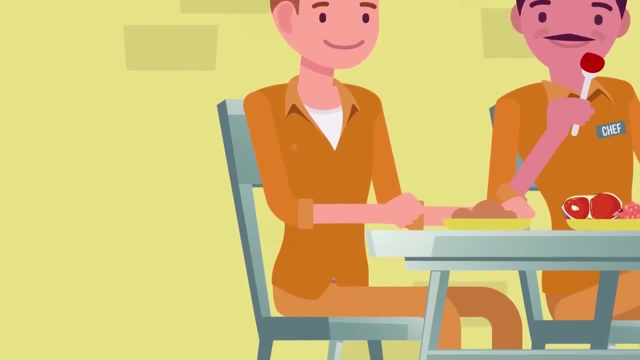 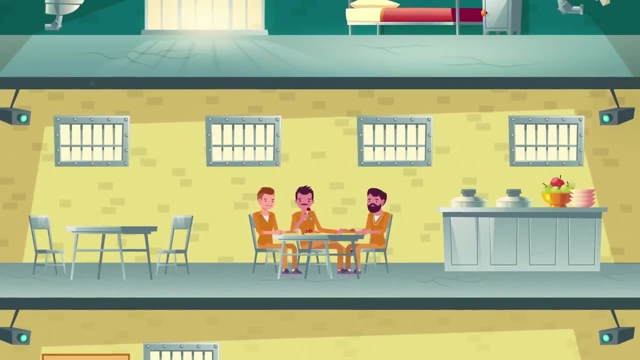 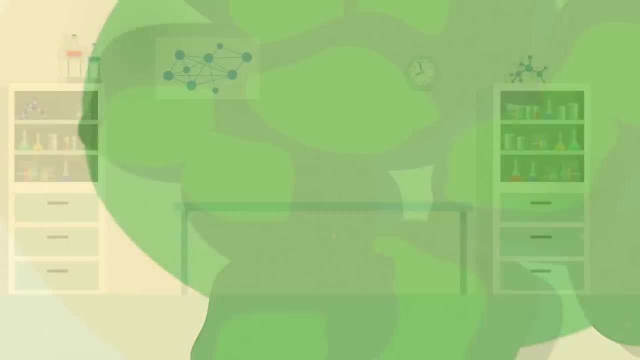 It's the third guy. Rich people try to keep low profile in prison not to be targeted by others. That's why he doesn't flash any valuable possessions or his status. A group of researchers is trying to test your knowledge. They take you into their lab on an island in Italy and present three dishes to you, but only one is safe to eat. 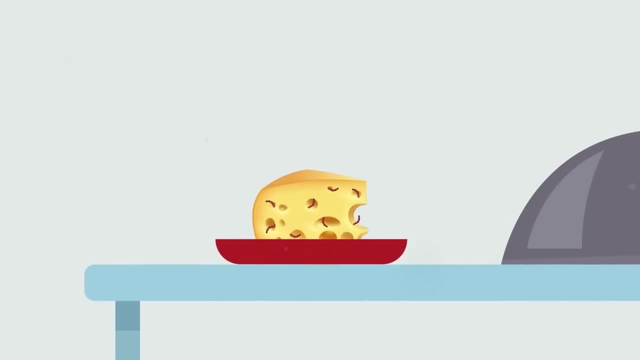 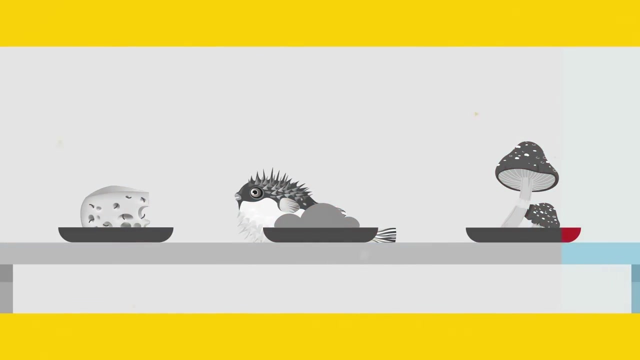 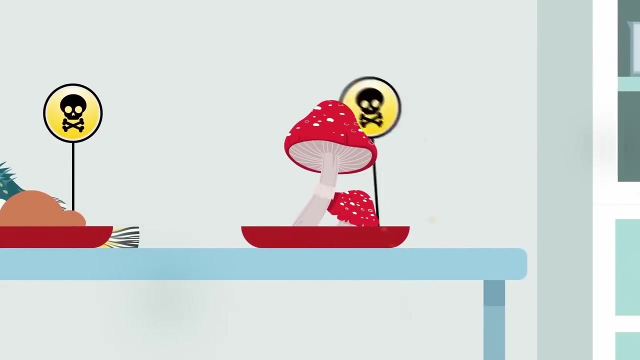 Which do you choose: Cheese infested by maggots, boiled pufferfish liver or fly agaric mushrooms? Pufferfish liver can be poisonous if it isn't prepared properly, and the fly agaric mushrooms are among the most dangerous in the world. 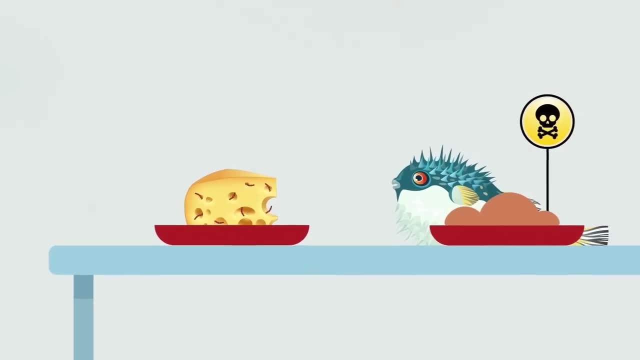 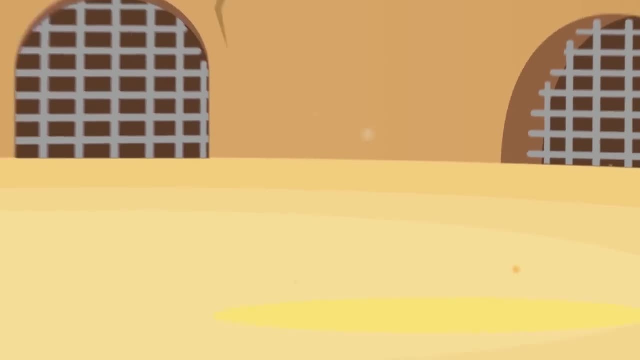 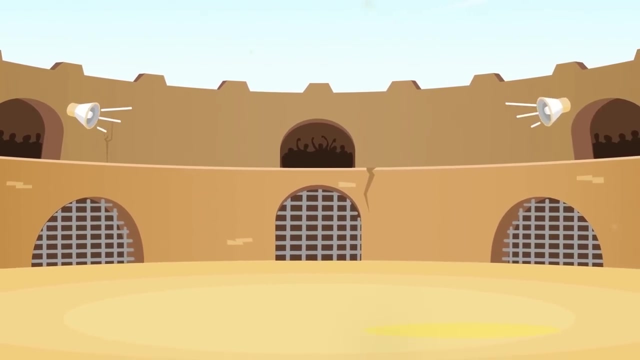 Maggot cheese, on the other hand, is actually a delicacy in Sardinia Italic, so it's perfectly safe to eat. Really, One day you wake up in an arena without knowing how you got there. From the speakers you hear that you must fight one of three hybrid animals. 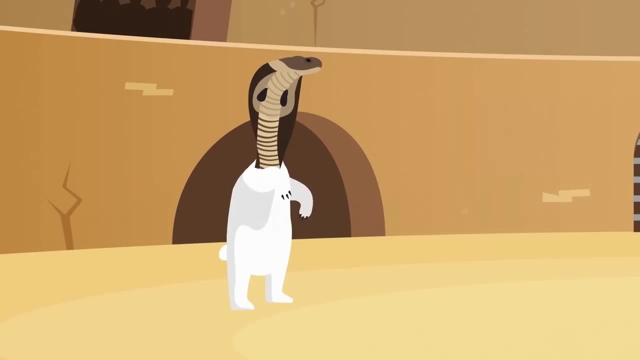 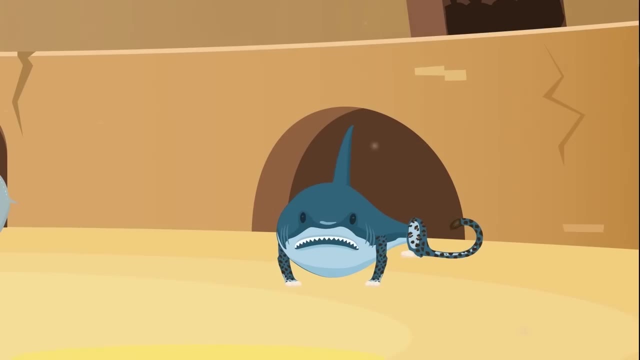 Which one do you pick to stay alive: A polar bear with the head of a rattlesnake, a hippo with a lion head or a hybrid with the face and body of a great white shark and the limbs of a jaguar? 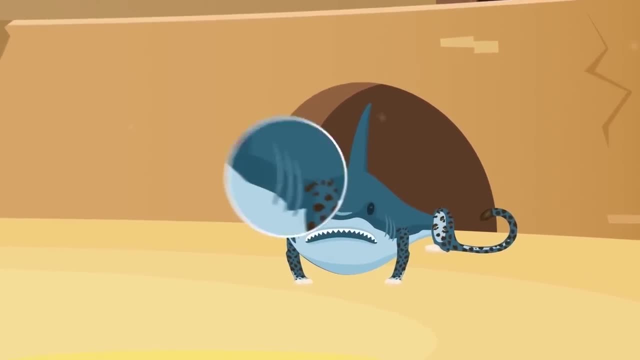 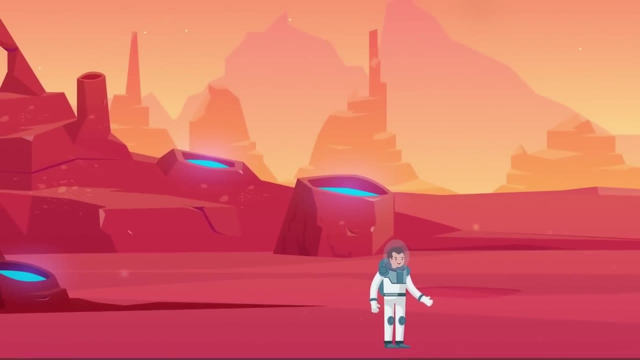 The great white shark hybrid. Since its body has gills, it won't be able to breathe outside water. You're an astronaut and you've made it to Mars for an expedition. A team member greets you at the entrance to the base in their workout clothes. 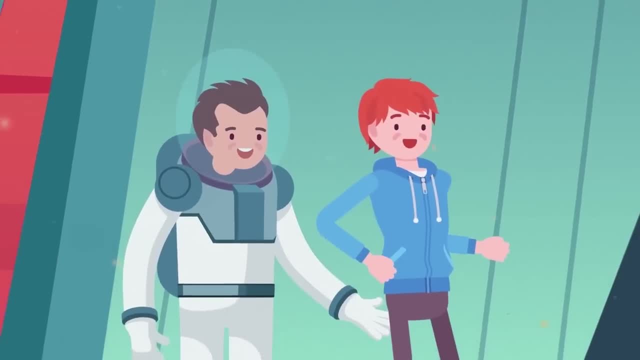 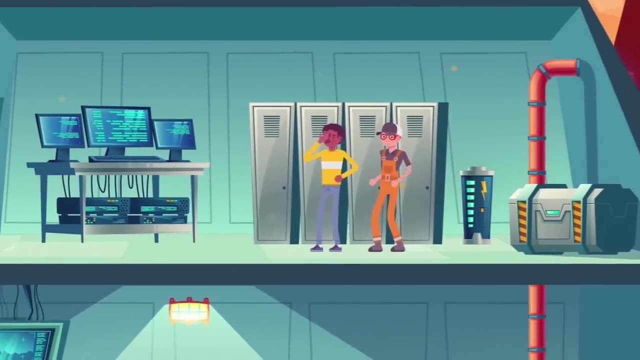 When you get in, you close the door and wait for the room to pressurize before taking off your spacesuit. When you walk in, you get a message that someone at the base is an imposter. Who could it be? A fellow astronaut who covers his face because he got a sunburn. 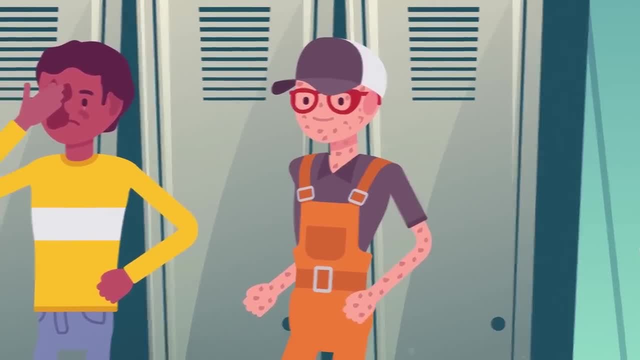 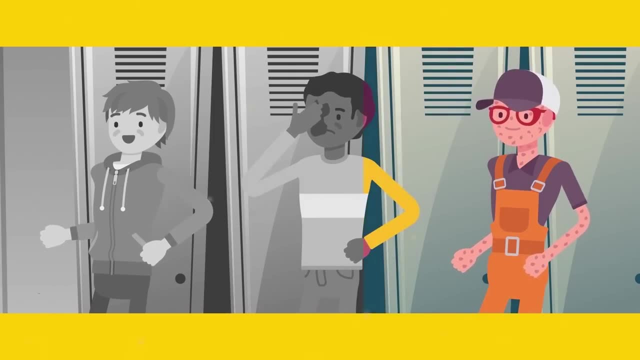 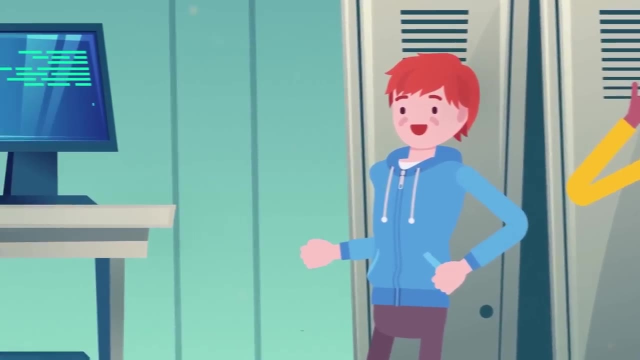 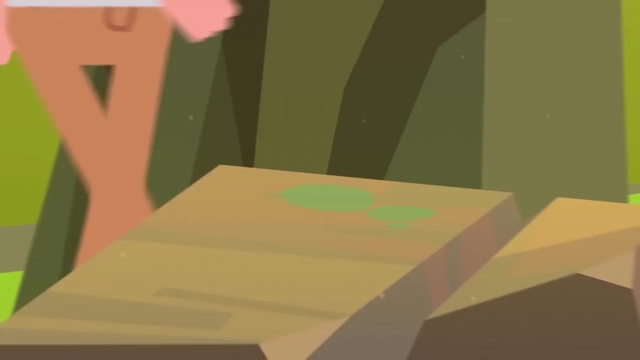 An engineer with flaky patches on her skin, Or the person who greeted you at the door earlier, The person you saw earlier. If they were human, they wouldn't survive outside the base in the planet's atmosphere. While walking in the forest, you come across a mysterious local that blocks your way. 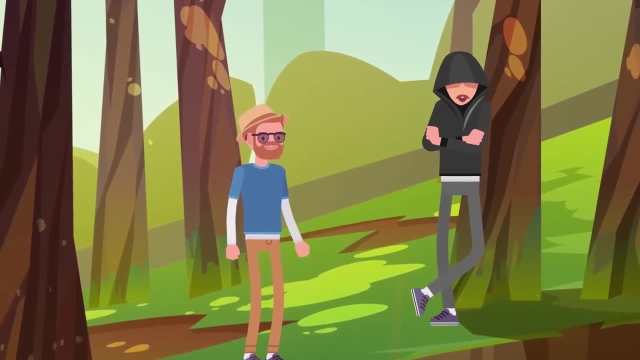 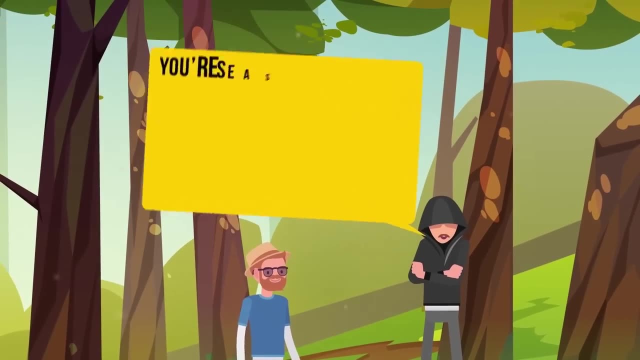 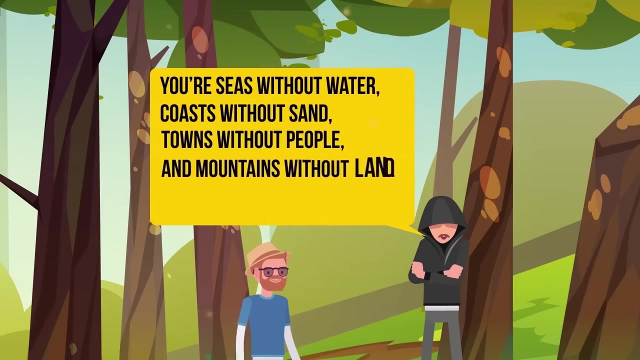 He tells you, if you solve his riddle, you're free to go, But if you don't, you'll have to stay in this forest forever. The riddle goes like this: You're seas without water, coasts without land, towns without people and mountains without land. 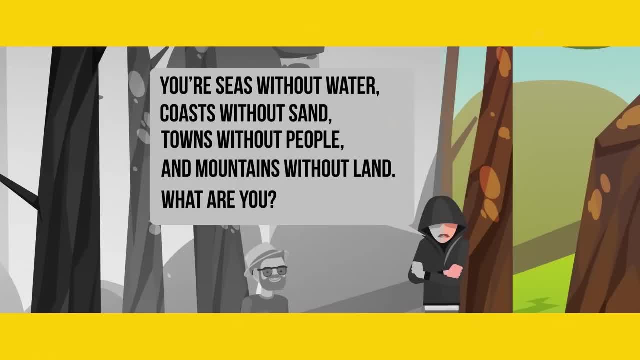 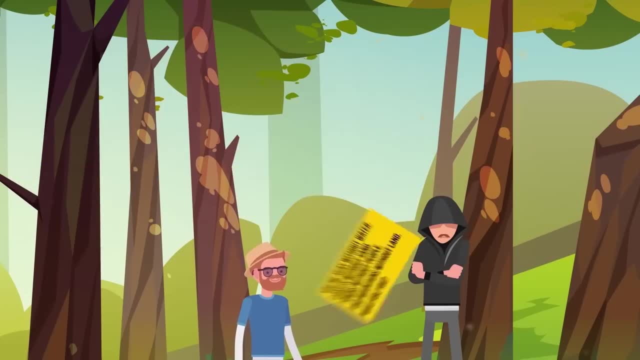 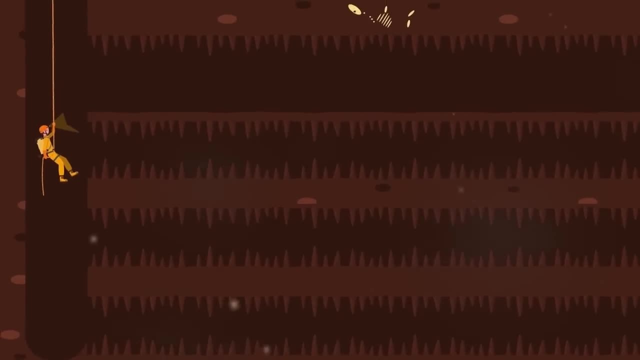 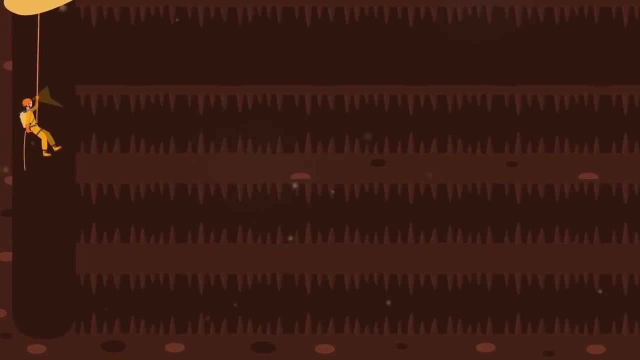 What are you? Well, you're a map. You decided to go exploring a local cave. You walk inside and a landslide suddenly blocks the way back Ahead. there are four tunnels, each with a sign showing you which dangers lurk inside. 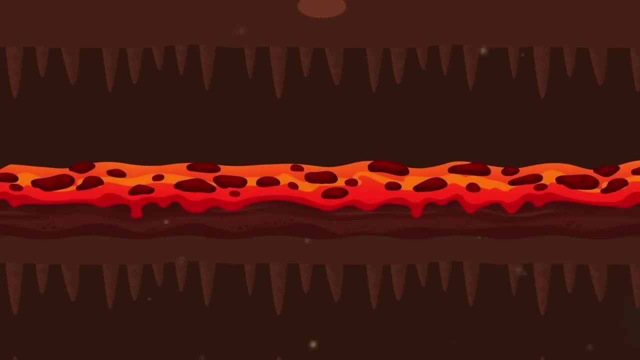 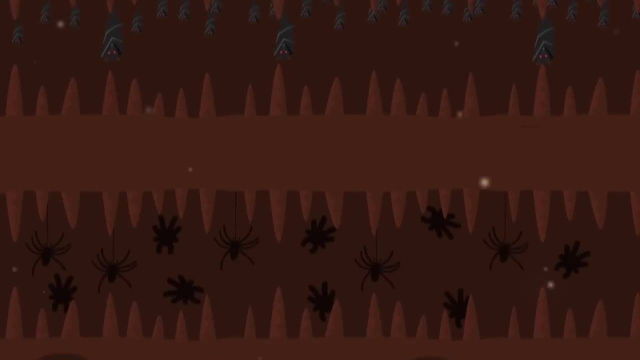 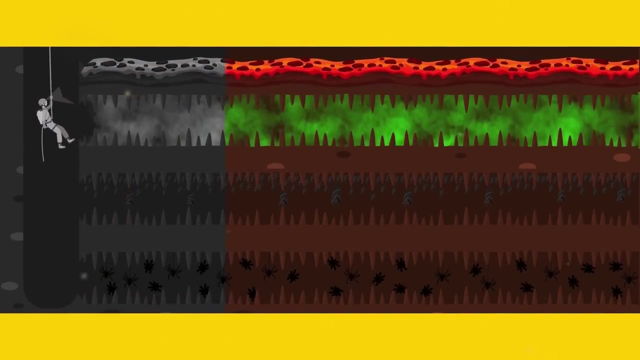 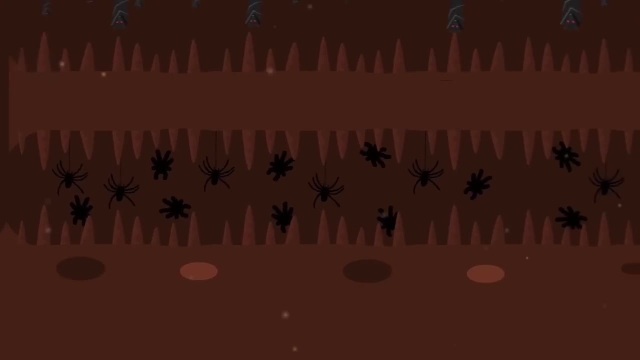 Which one do you choose to stay safe? The tunnel filled with molten lava, the one filled with poisonous gas, the one swarmed by bats or the tunnel with venomous spiders? You picked the last one. Spiders don't hunt humans for food and usually avoid them altogether. 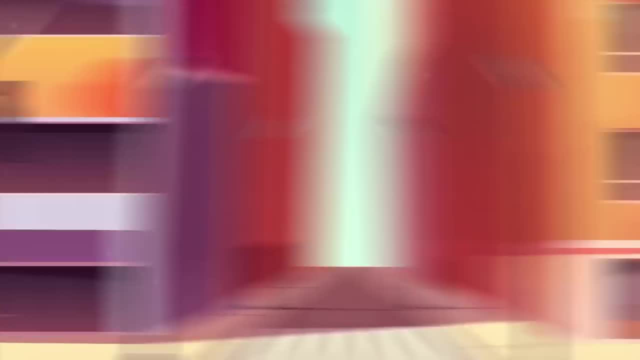 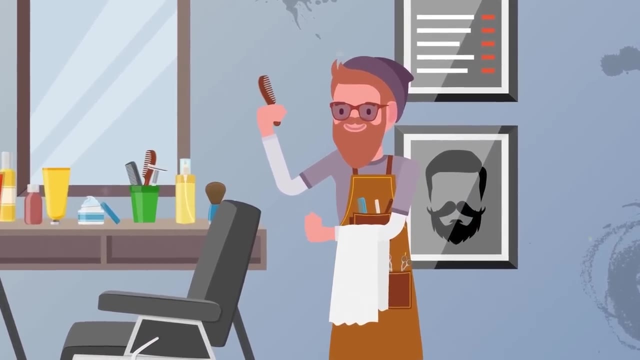 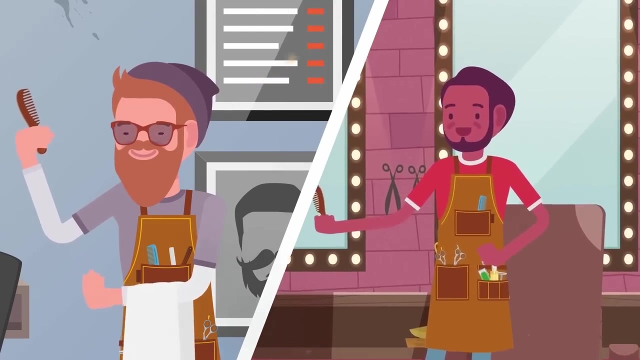 You just moved into a new town with only two barbers. You visit both their shops to decide which one you should pick. The first shop is a bit messy and the barber needs both a haircut and is beard-trimmed. The second shop is shiny, tidy and the barber is well-shaved with a perfect haircut. 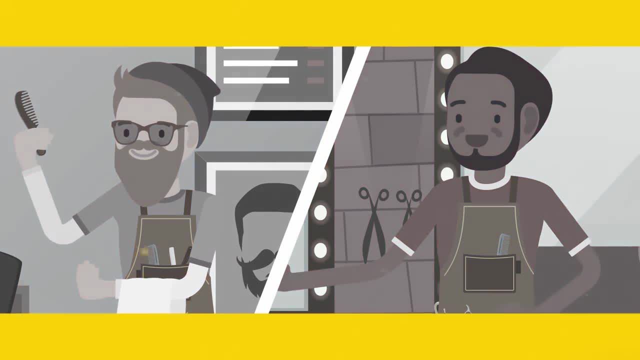 But you decide to go to the first shop. Why? Because the barbers don't want you to go to the second shop and the barbers don't want you to go to the third shop. The barbers don't want you to go to the third shop and the barbers don't want you to go to the fourth shop. 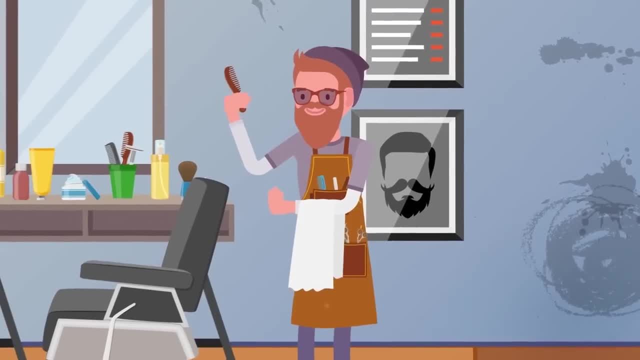 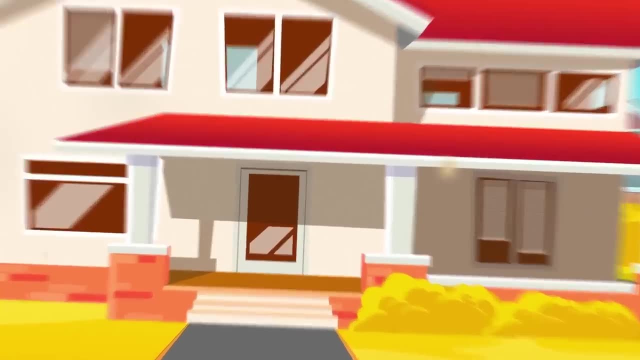 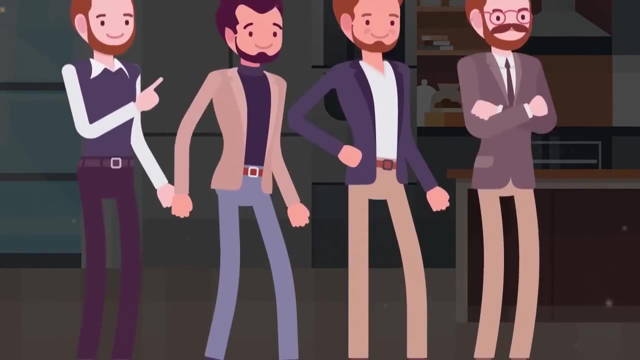 Each barber cuts the other barber's hair and you pick the one who gave the other a nice haircut. You've got a job as a helper to someone's mansion, but the mansion owner gives a tricky task. I need the least number of chairs for a table to seat four fathers and two grandfathers with four sons. 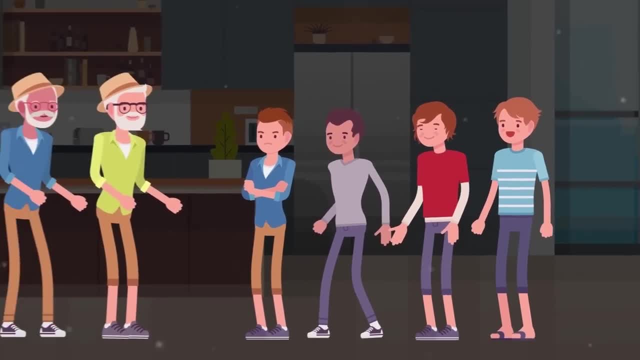 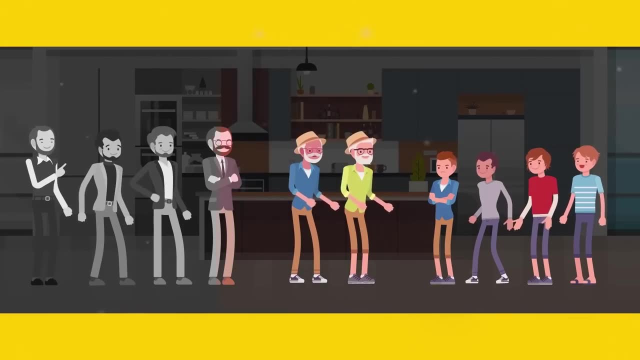 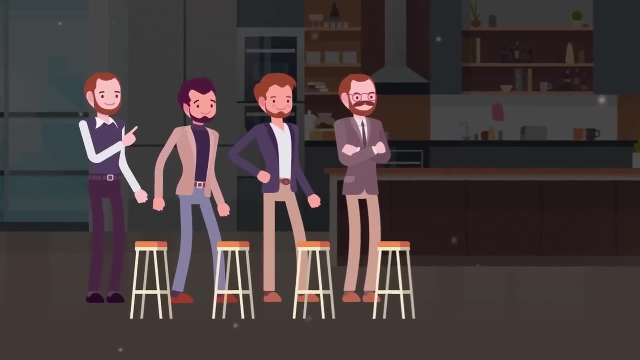 You can't ask anyone to help you. You can't ask any questions. but what's the least number of chairs? you must put out Four. The fathers could also be grandfathers and they're all sons. Mary was selling a rope for $3..